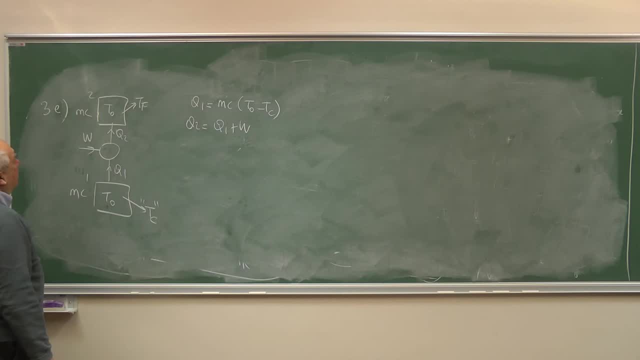 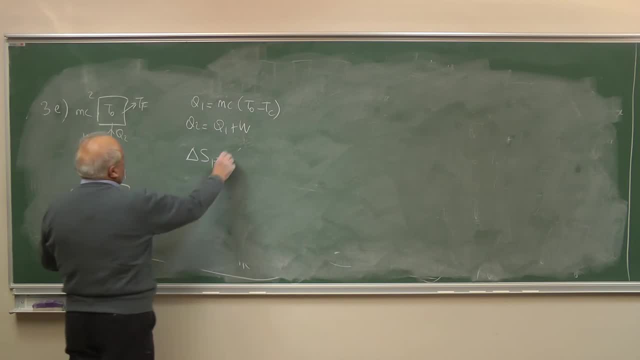 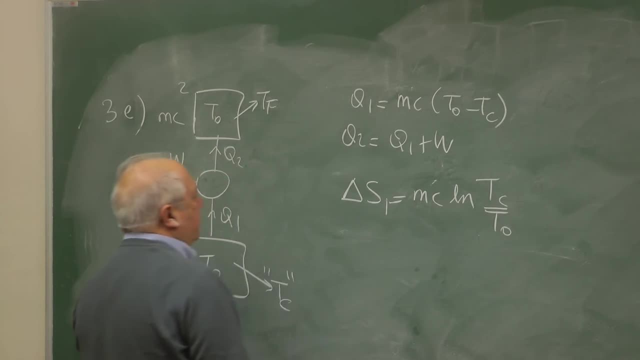 Delta S1, that's equal to Mc log Tc over T0.. Delta S engine: that's equal to zero, Because every time it was doing a cycle. delta S2 is- it's not a reservoir. so we are putting it bit by bit, keeping it in equilibrium. 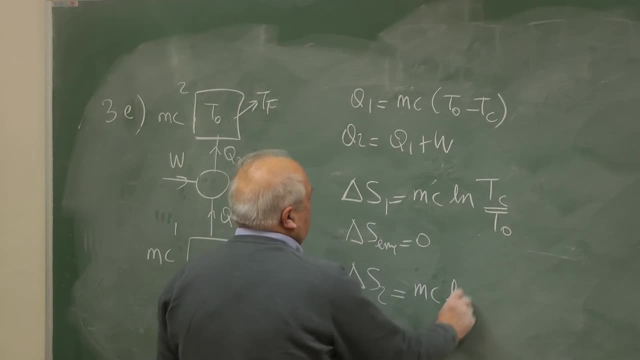 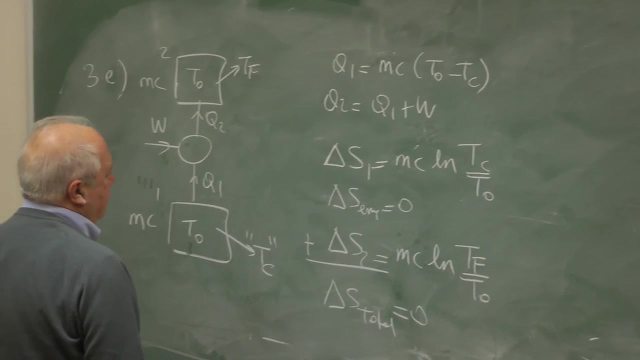 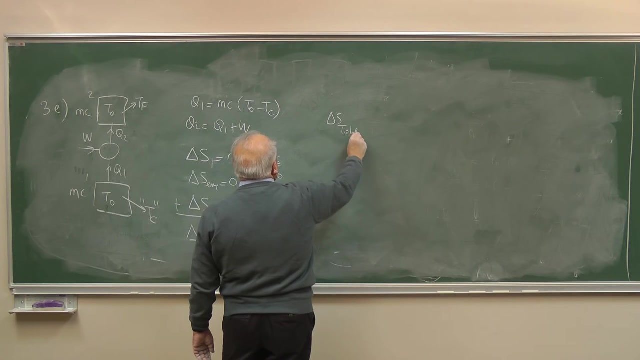 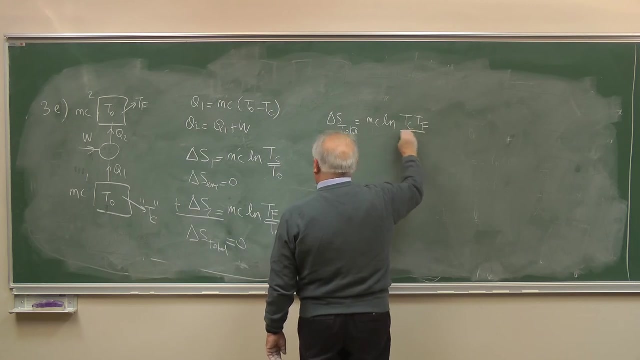 So it is MC log. finally, TF starting from T0.. So the totality will be 0, delta S total, So delta S2.. So delta S total equals MC log: TC TF over T0 squared. 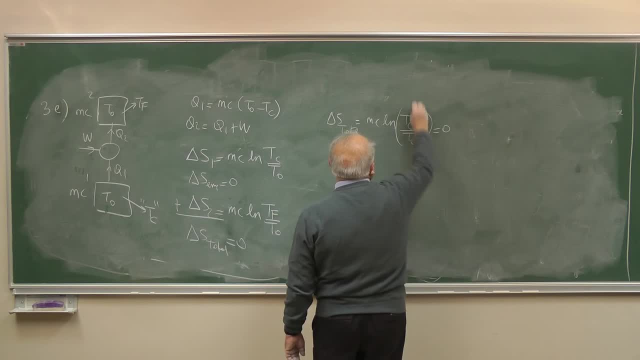 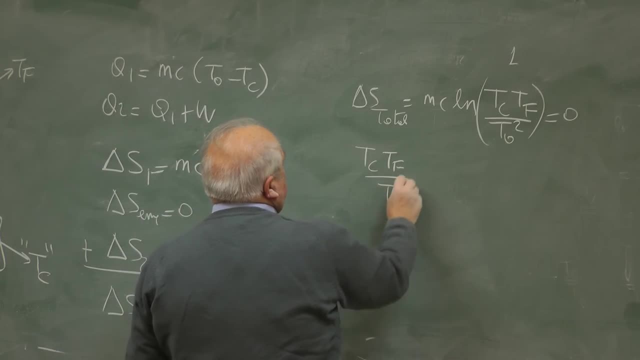 So this must be equal to 0.. That means the log term must be 1.. TC: TF over T0 squared is equal to 1.. TC is known, it is given. We were given TC. So the final. how hot will this get? 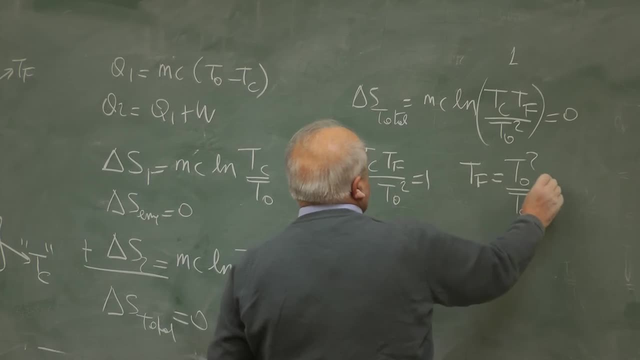 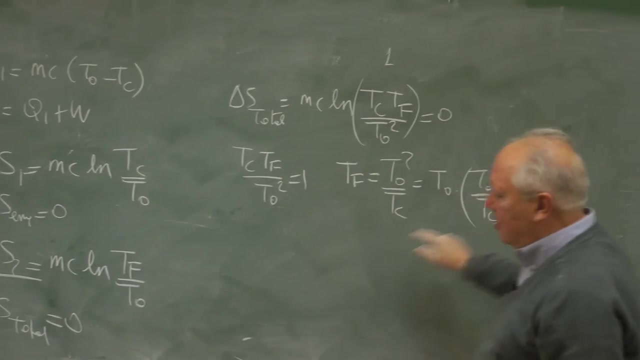 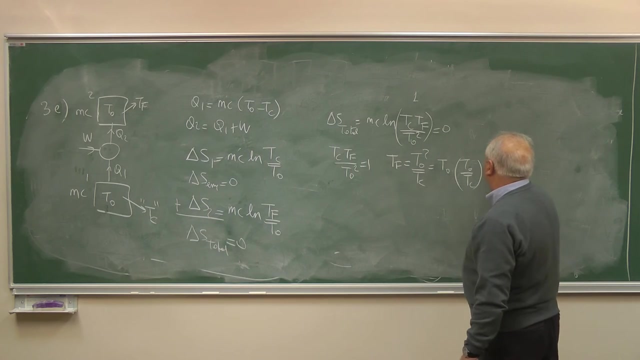 This is T0 squared over TC, which we can write T0 times T0 over TC. Since T0 was the higher temperature, we lowered the temperature to the colder temperature, So this ratio is larger than 1.. It means TF is, as expected, larger than T0.. 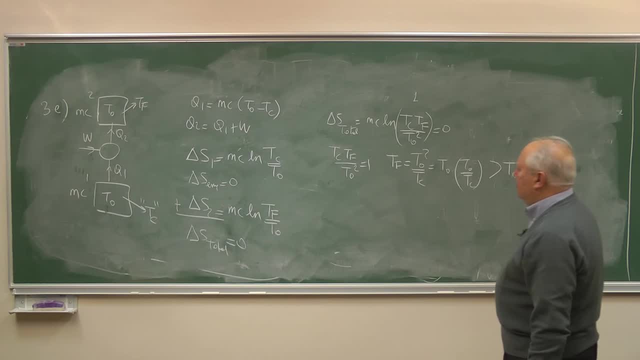 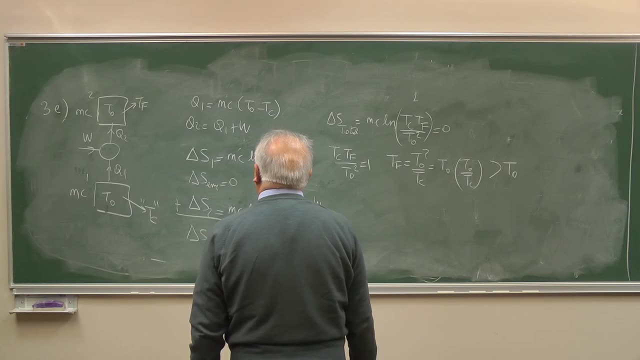 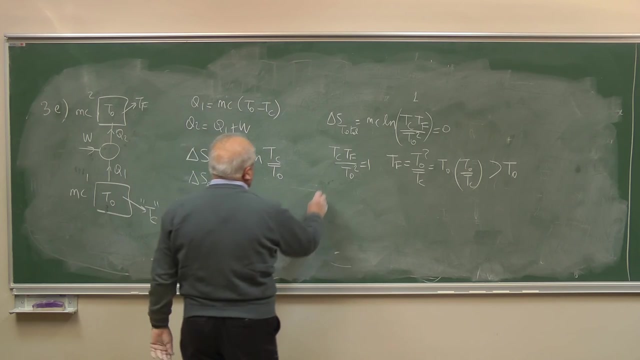 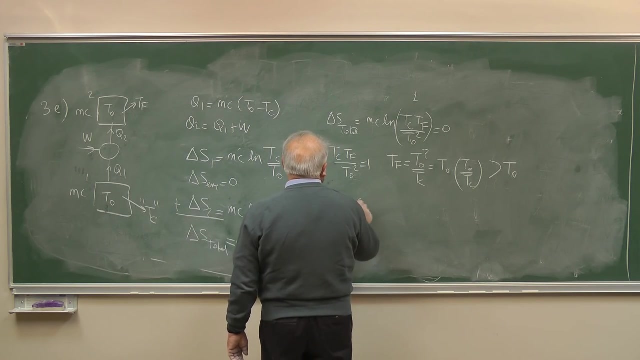 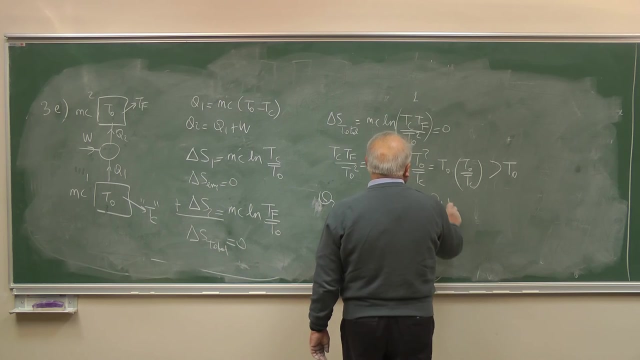 So what is W? Q2, we also know, because Q2 is the amount of heat that raised its temperature from T0 to TF. So Q2 is equal to MC Tf minus T0, which is Q1 plus W minimum. Q1 is MC T0 minus TC plus W minimum. 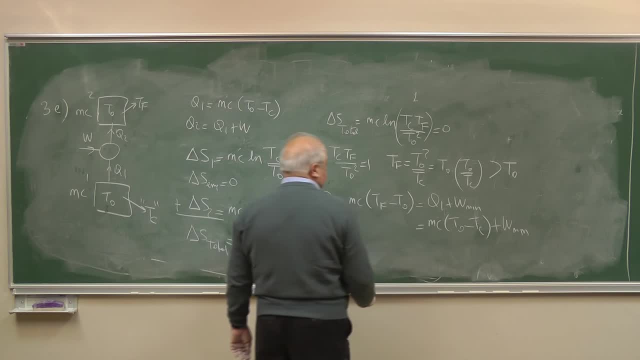 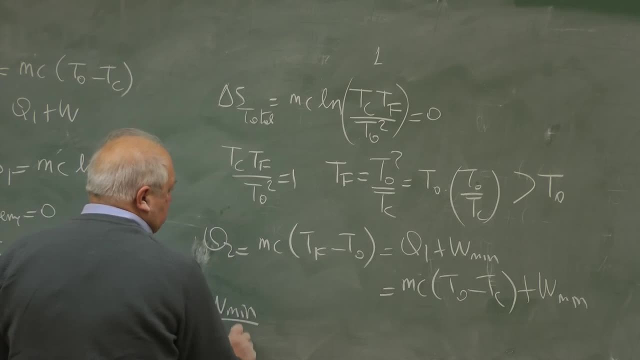 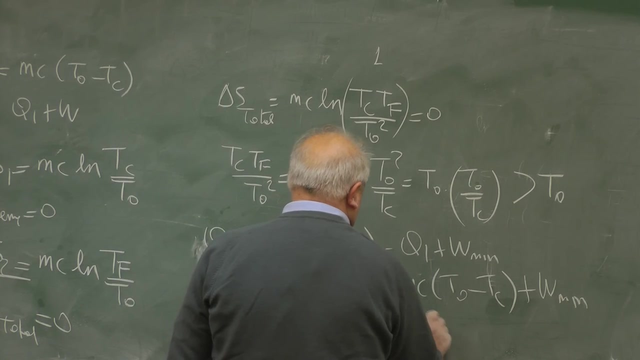 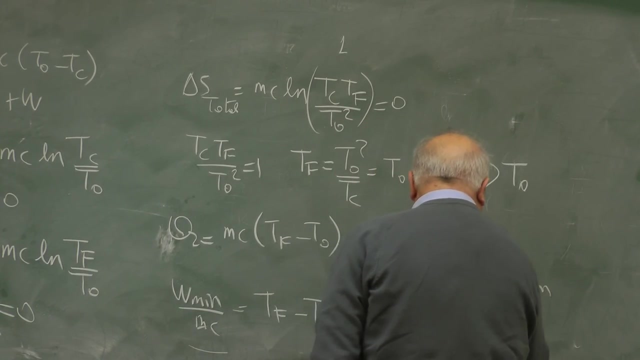 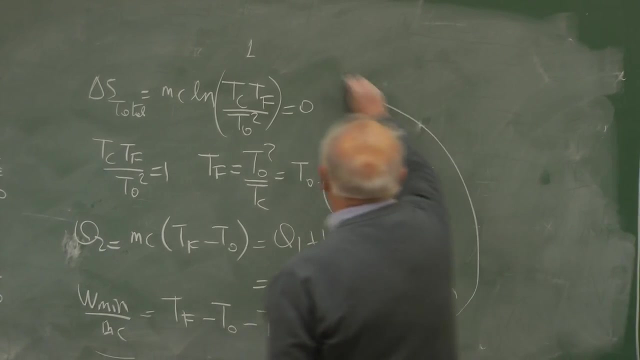 Therefore, W minimum over MC, MC. if I divide everybody by MC, that's equal to TF minus T0 minus T0 plus TC, which is TF plus T0 minus TF plus TC over 2. T0. T0. Tf is T0 squared over TC. 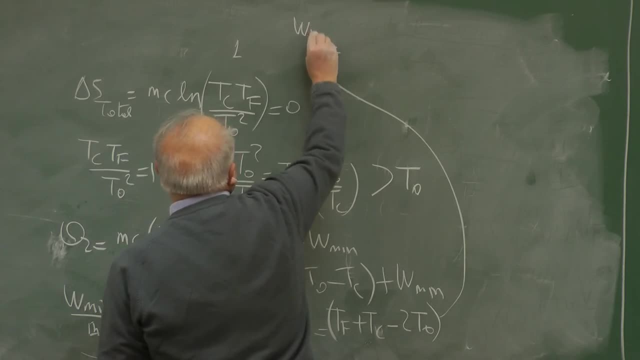 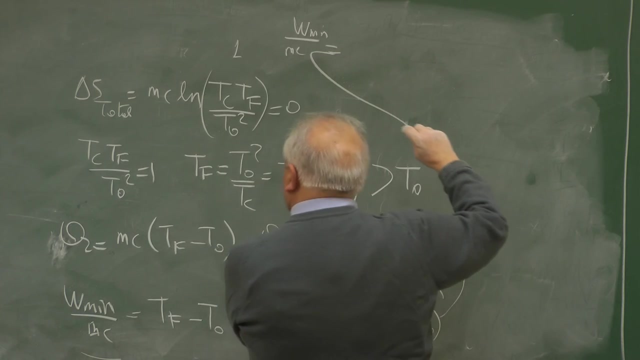 So W minimum over MC is equal to TF. is T 0 square over TC plus TC minus 2 T 0. I multiply by TC and divide by PC, so it is T 0 square minus 2 T 0 TC plus T C square.